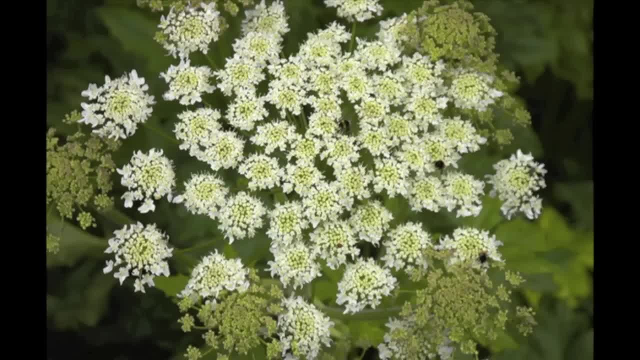 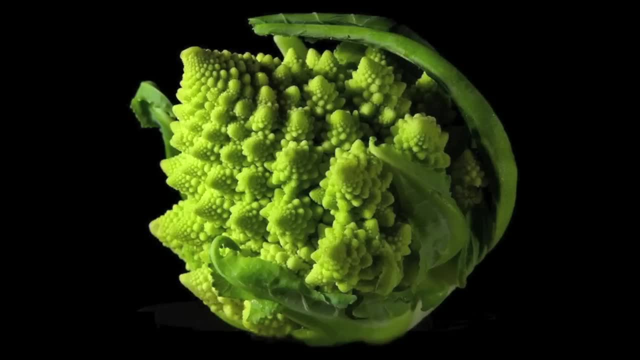 is, in fact, similar to each of the flowers and even to the bunch. This is also an example of a fractal pattern. Another fractal is a broccoli- And don't we all really love broccoli? As you can see, each of the heads of the broccoli resembles a vegetable as a whole. Now that you've seen these examples, 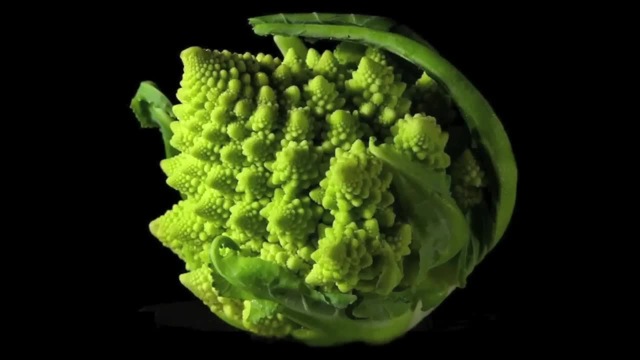 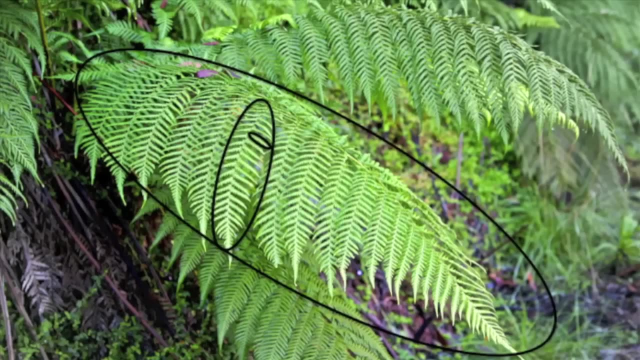 of fractals. you can probably spot your next fractal in nature by yourself. So what exactly are fractals? The word fractals comes from the Latin verb to break. Fractals are geometric patterns in which every smaller part of the structure is similar. 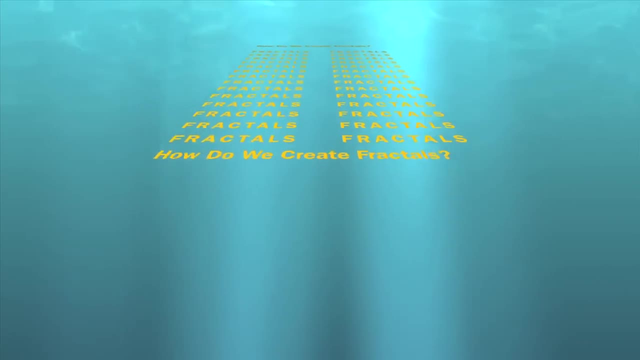 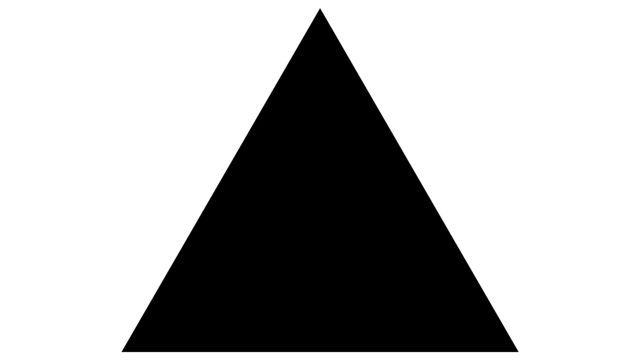 to the whole. How do we actually create a fractal? Let's first look at the Sierpinski triangle. It does look complicated, but we can create this in a few simple steps. Let's start with the black triangle. We can mark the center of each side of the triangle and 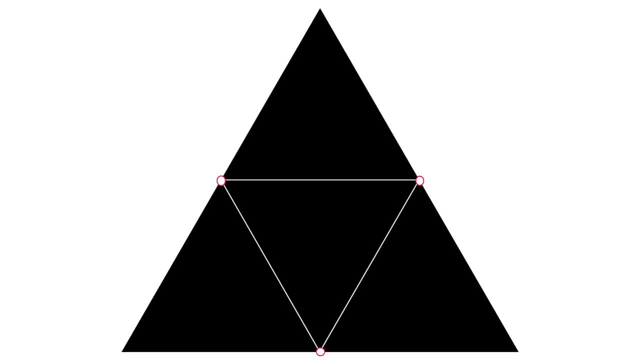 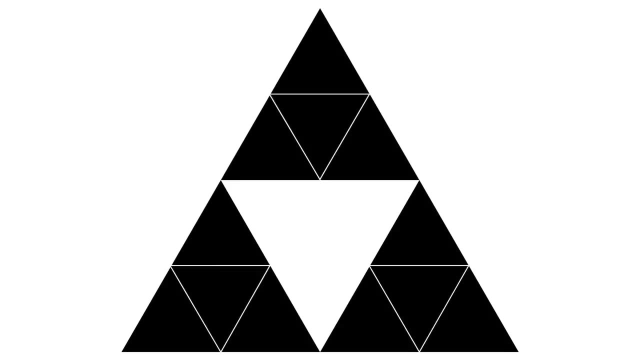 connect the dots to make a new upside down triangle. We then remove this triangle and are left with three smaller black triangles instead of one. Let's remove the three new triangles and again connect the dots to make three new upside down triangles. Let's remove the upside down triangle at the top. Look, we get three new. 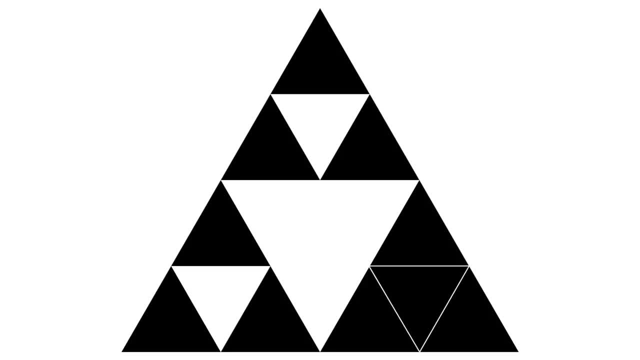 triangles. instead of the one at the top, We can now remove the one at the bottom left and finally the one at the bottom right. You'll notice that each time we remove an upside down triangle, we get three new black triangles, So now we have a total of nine, even smaller. 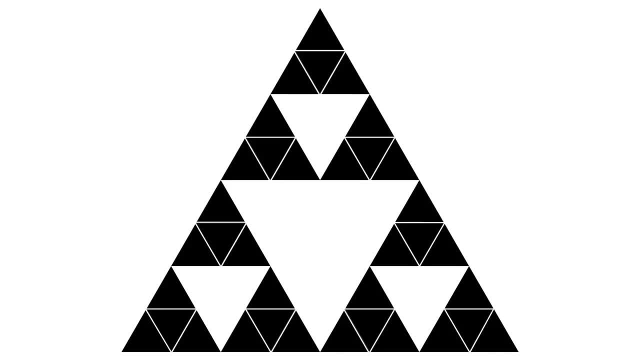 black triangles. Let's see the triangles that we will remove in the next step. Now we can again take the top part of the big triangle and remove the upside down triangles. We can continue on to the bottom left and then the bottom right. We already have twenty-seven. 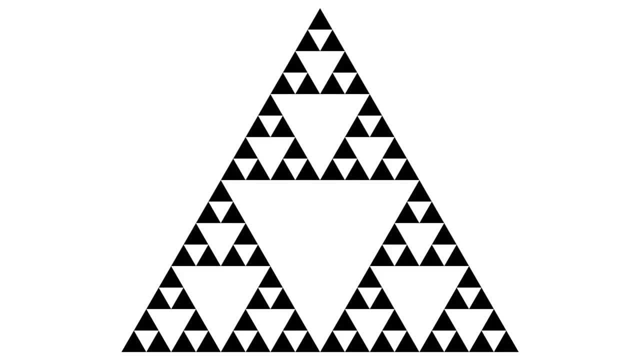 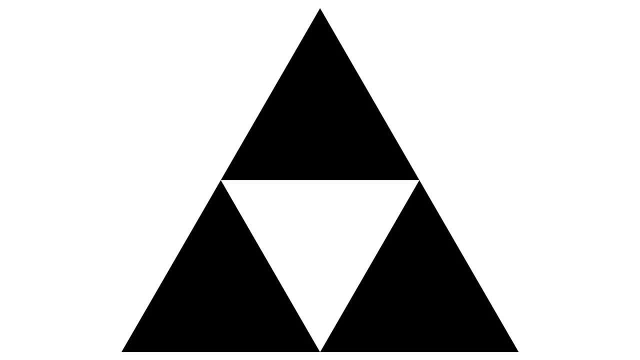 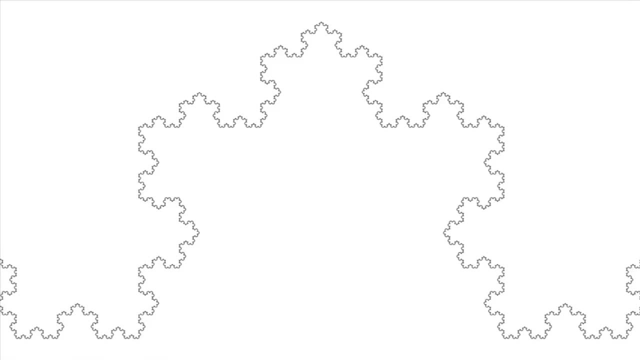 black triangles. If we keep going, we can make more and more black triangles at each step, And if we keep doing this forever, we'll have an infinite number of triangles, and all inside the one big triangle we started with. Let's have another example. This one is called the Von Koch curve, named after the Swedish 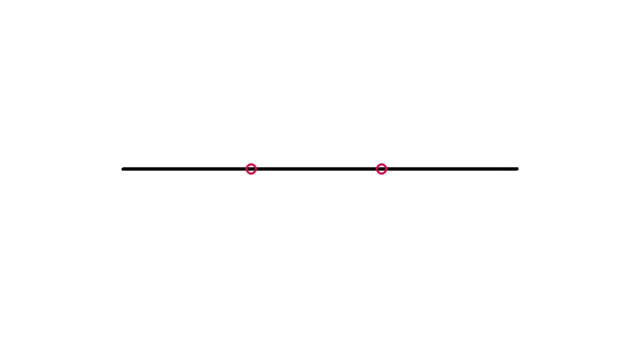 philosopher who came up with it. This time we start with a line and divide it into three. We mark these points, then take out the middle. We take a line of equal length to the one we just removed and put it at an angle of sixty degrees. We can now connect the two.